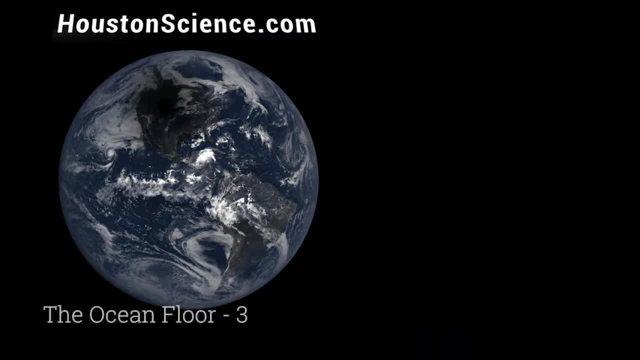 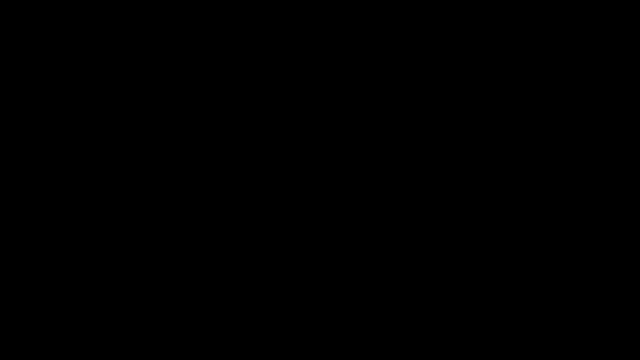 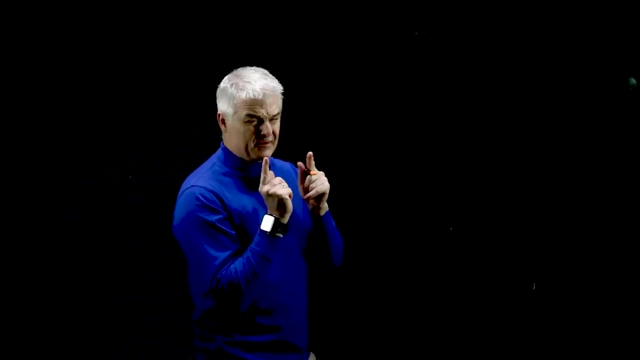 Okay, Houston, we've had a problem here. This is Houston. say again, please, Uh, Houston, we've had a problem. Houston, no problems. We're studying the depths of the ocean, The deep, deep parts of the ocean. 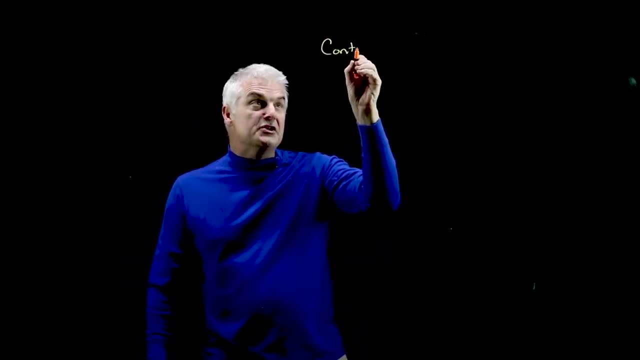 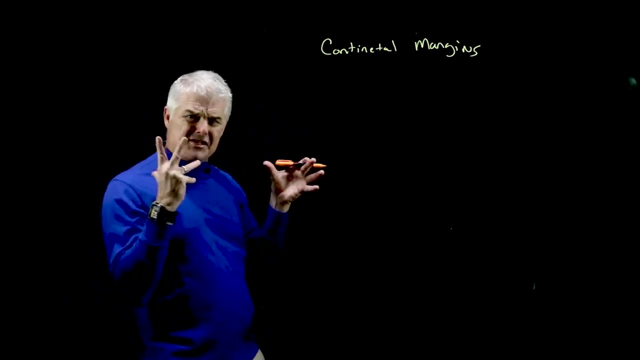 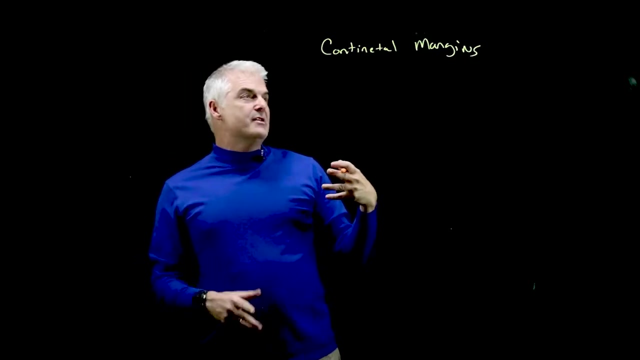 And what we want to learn today is about the Continental Margin. Seriously, folks, when we look underneath the ocean, we see cool, crazy stuff. Remember last video we said we're going to break it into three parts: Continental margins, the deep part of the ocean and the ridges. 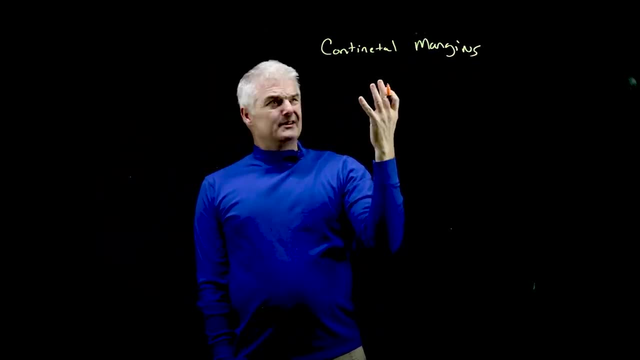 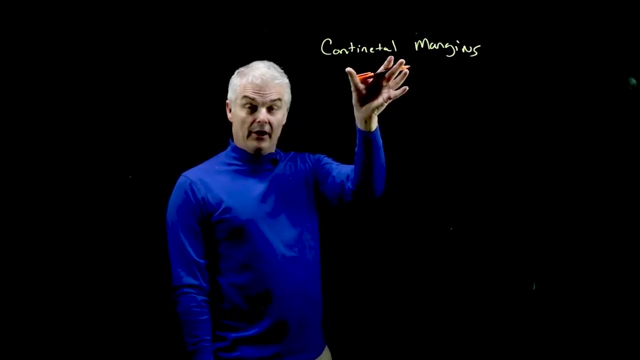 Today, continental margins. So what's a continental margin? Well, you know what a margin is right: The margin of a piece of paper. It's the edge. So the edge, the margin of the continent. Take a look at the picture here. 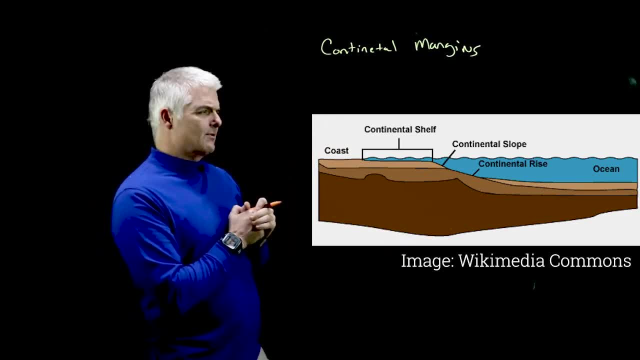 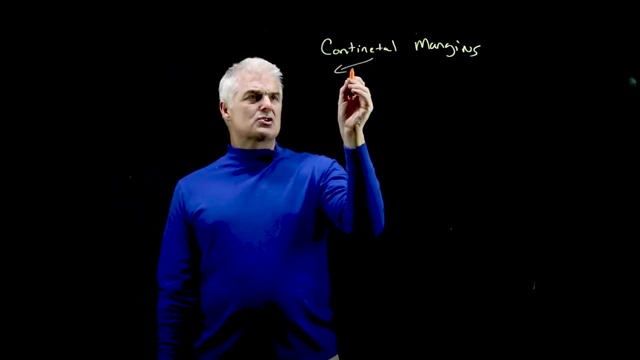 Pretty cool. You can see interesting features in the image of the continental margin And we want to talk about what they are. Now it turns out when we talk about the continental margins there's two types of continental margins. The first one is called passive. 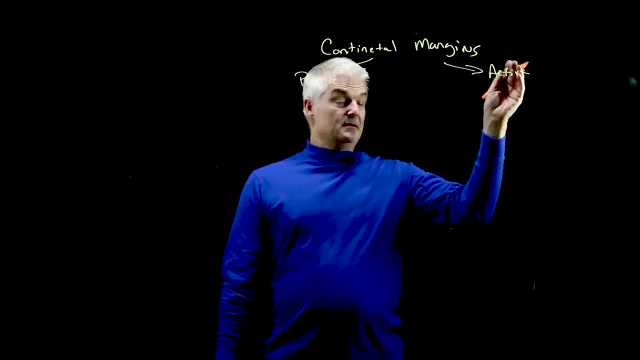 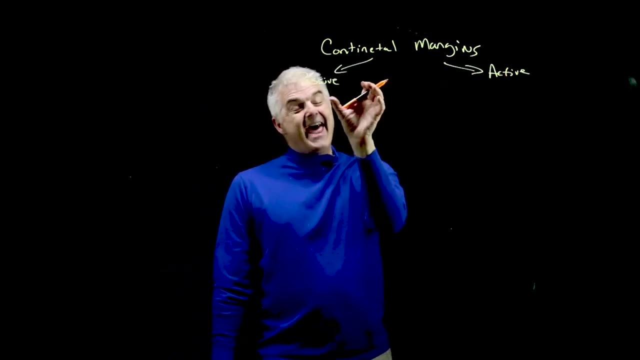 And the second one is called active. Make sense, Passive-active. Now, active ones mean active from a plate tectonomic, tectonomic Tectonic perspective, And the passive ones where there's not a lot of super plate tectonic things happening. 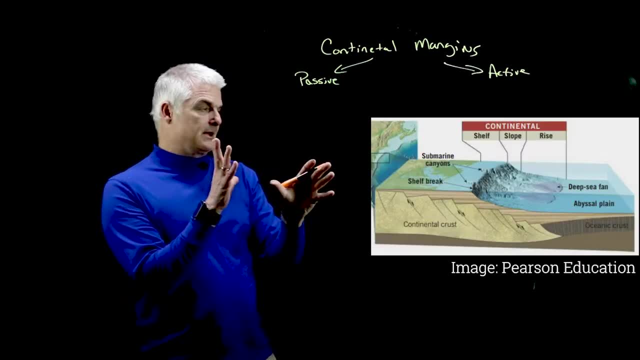 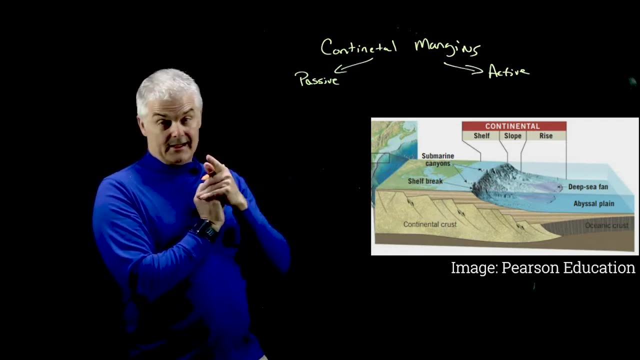 So let's start with passive first. So when we look at a passive plate boundary- All right. so this is a plassive, plassive, Passive plate boundary. There's a number of features that we want to highlight, So let's dive in. 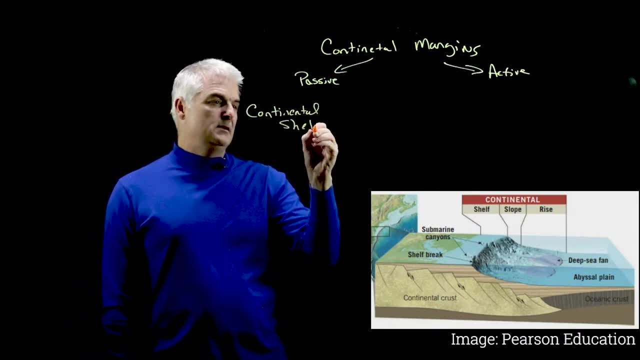 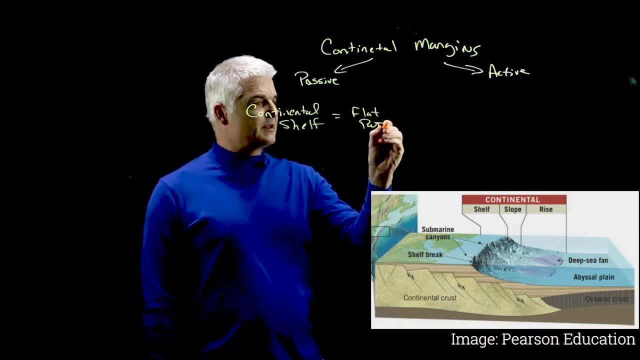 The first one is the continental shelf. So you can see that right here. So the continental shelf is what do you say? That would be the flat part. So at the edge of most continents, P-A-R-T. You'll see a flat part. 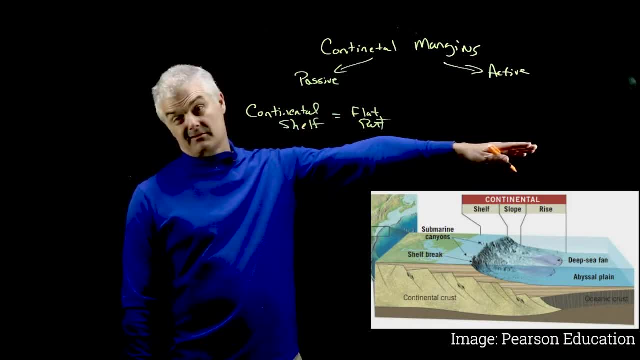 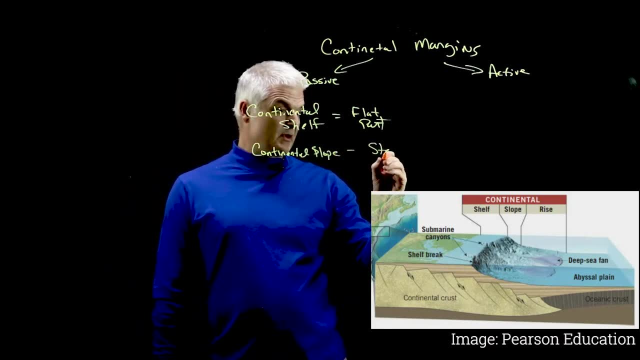 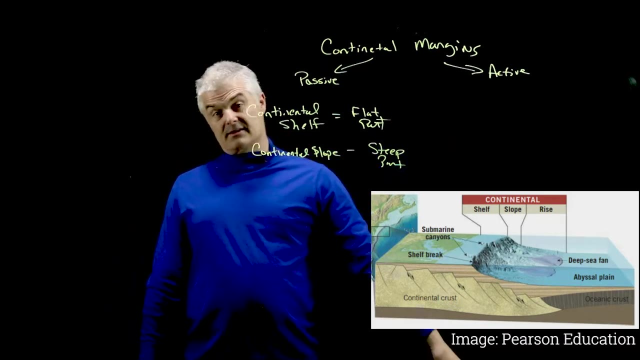 That's the continental shelf. Make sense, Looks like a shelf. The second one is the continental slope And that would be the steep part. You see that over there. So the actual continent actually sort of extends into the ocean And then it dives deep down. 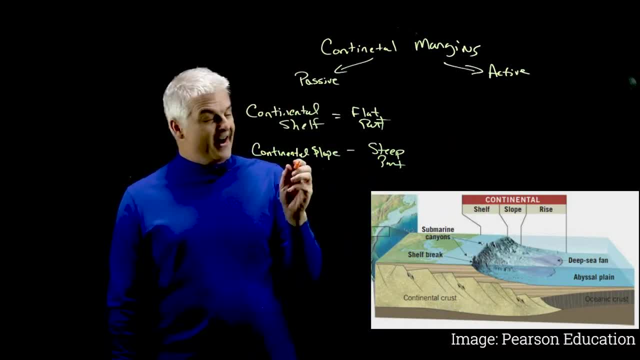 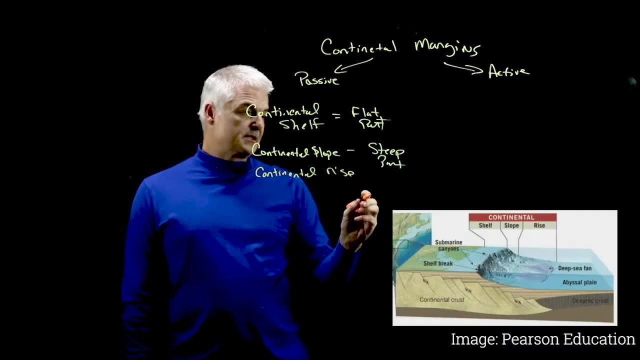 Down, deep, down, deep in my soul, And sorry. And then, of course, there's also just a gentle slope up And that's called the continental rise. And that's the shallow part. Yeah, It's still got a steepness to it. 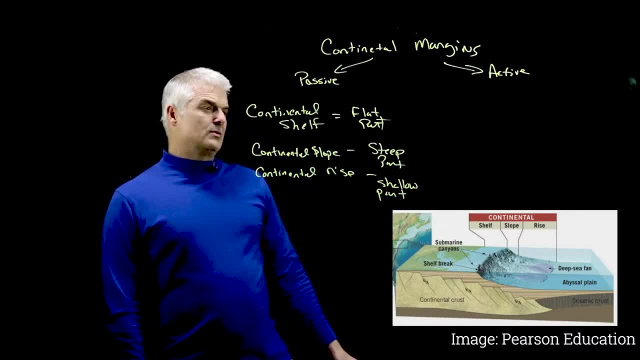 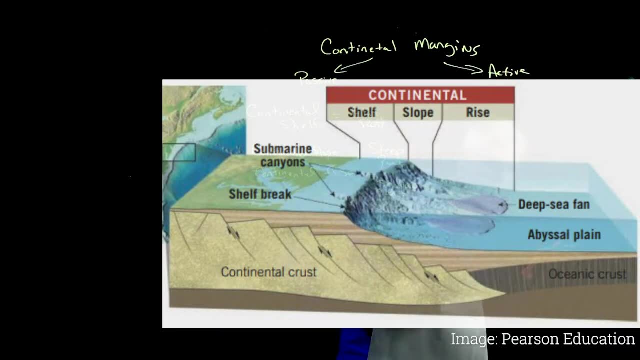 But it's not as steep. You see that, And so those are the big sort of three, But you might notice there's some weird things going on in this picture. So look at your picture. Ah, looking, And I see something strange there. 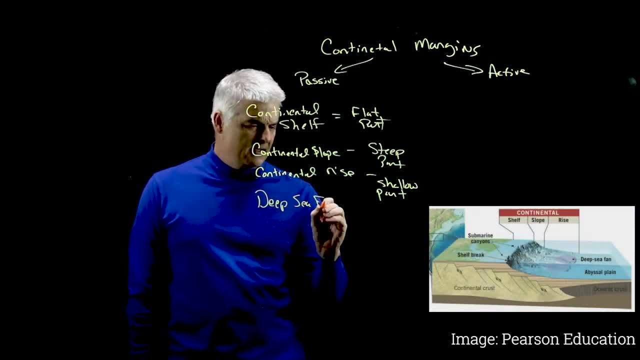 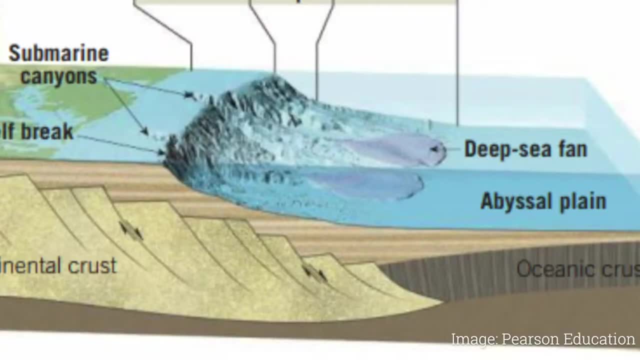 What do I see? I see a deep sea fan. All right, You can see that deep sea fan And it looks like something we've seen before When we were studying mass wasting, all this stuff we see on the edges of big oceans. we see an alluvial fan. 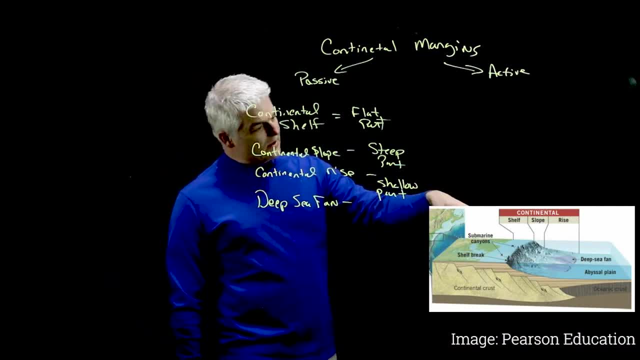 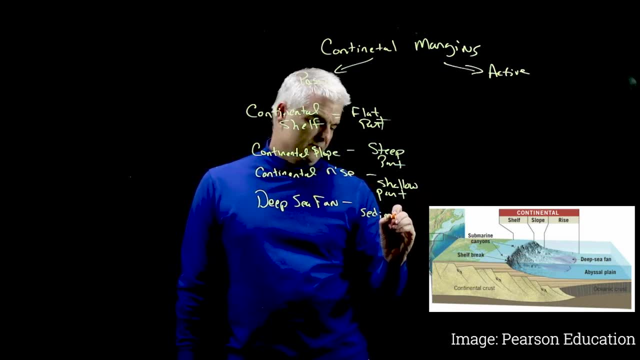 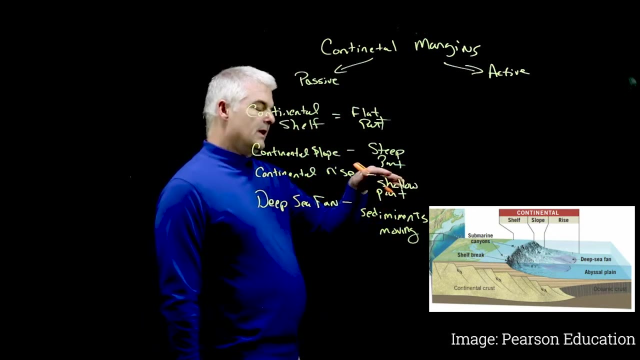 So this looks like an alluvial fan, But it's like an alluvial fan underneath the ocean And it's really caused by the same thing. What's causing the deep sea fan is sediments flowing downwards, Sediments moving. You see how the sediments are moving and they go down. 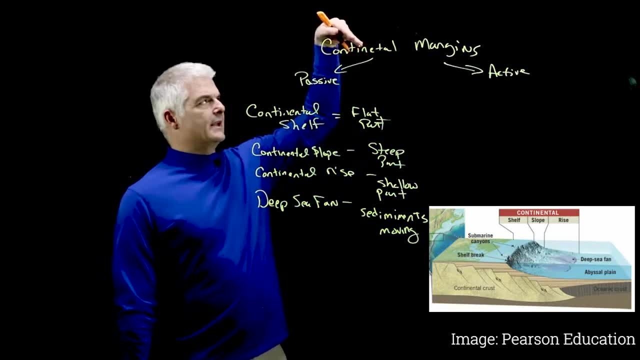 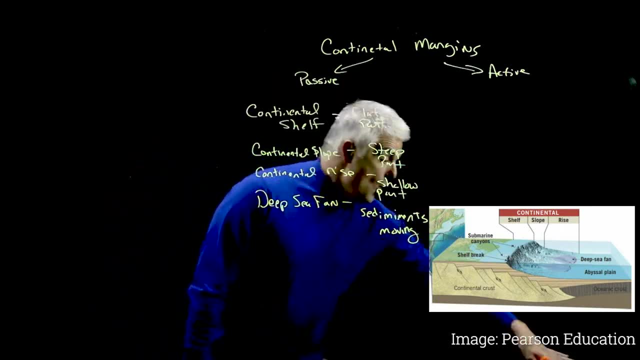 But there's something weird, because this is all happening underwater. right, It's not on land and it finally makes its way to the water. This is all underwater, But basically gravity is solving this or causing these things to happen. Flows down and makes that. 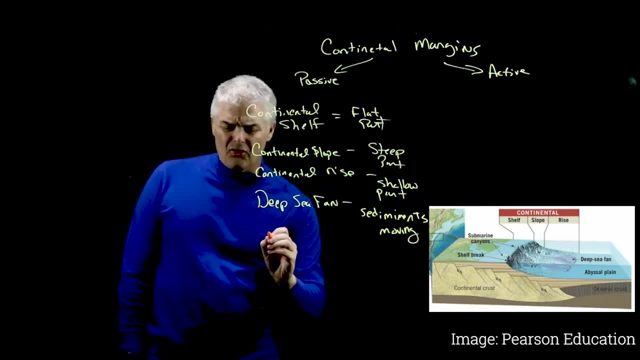 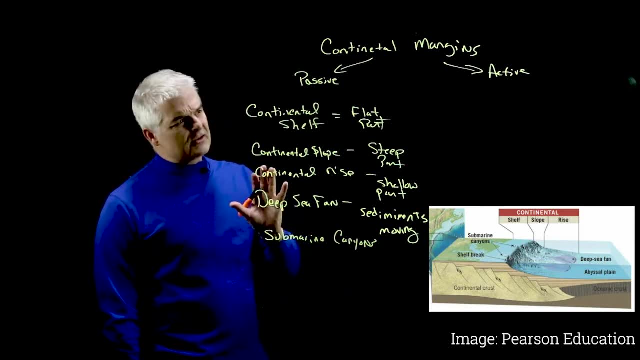 And in doing that you make these cool term. I love these things: Submarine canyons, Submarine. I know when you think of a submarine, you think of that, But what I'm thinking about is a canyon Underwater. 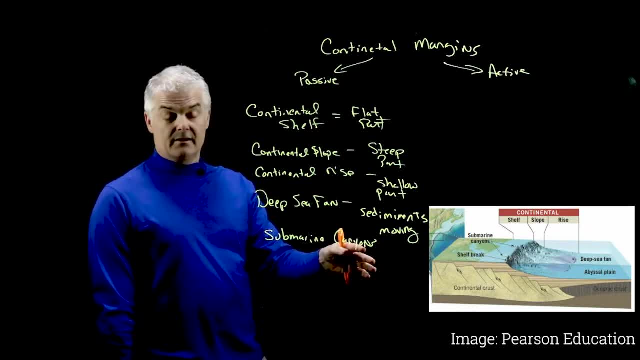 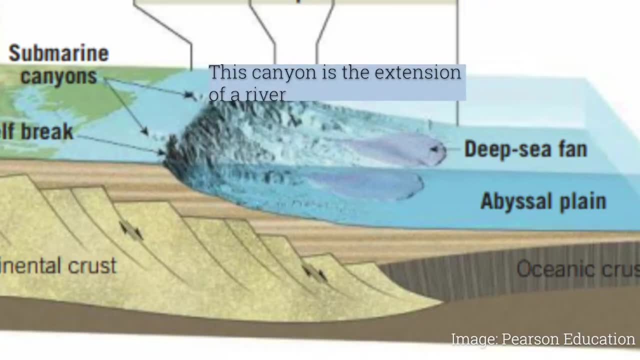 Sub, Under Marine Ocean, Under the ocean, A canyon, And these submarine canyons are caused by. Well, if you look back to the picture, it's going to be caused by a river. You see how the river flows out from the gland and then it flows out. 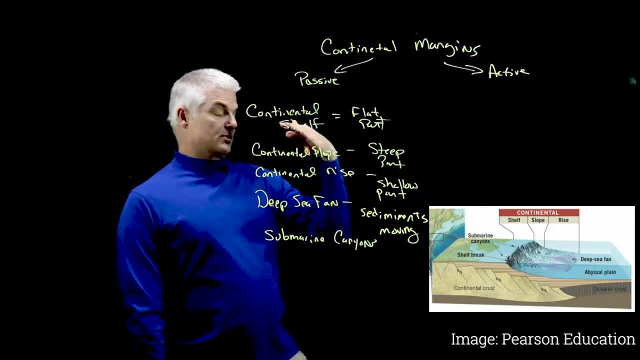 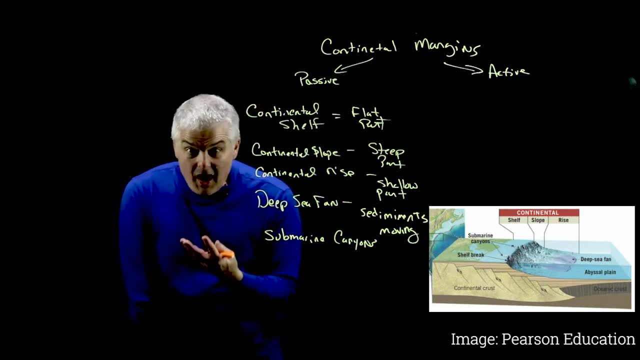 So we live near Galveston, Texas. There's a big river Flows through us. All that water has to go somewhere into the Gulf of Mexico. There's submarine canyons out there caused by the sediments flowing from us. 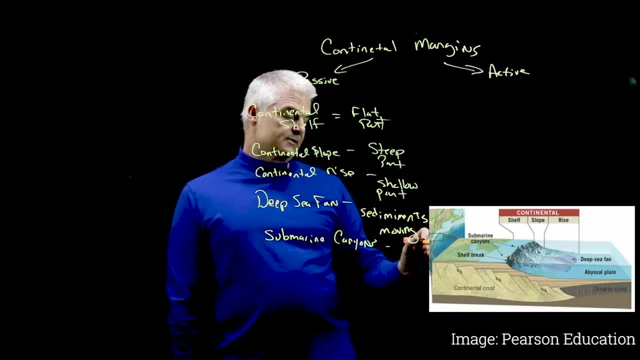 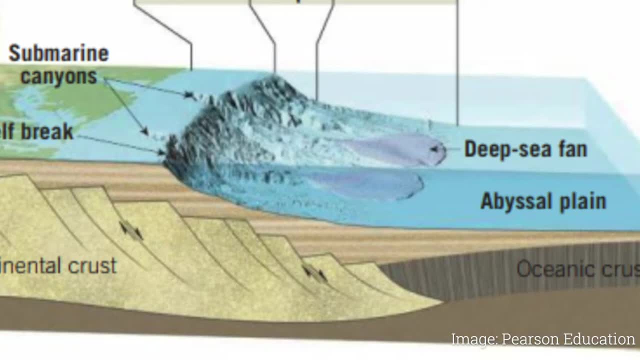 From us here in Houston- Submarine canyons. But if we look at the picture some more, I think you've seen it. There's one submarine canyon but there's no river that it's coming from. Do you see that? 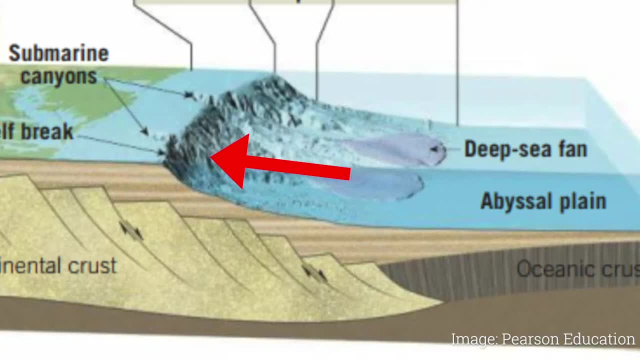 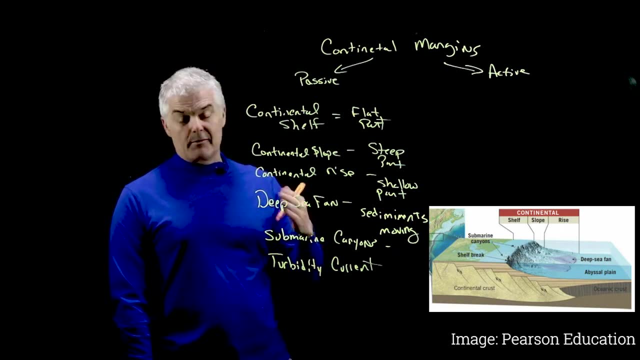 Isn't that weird? What's up with that? Where does that come from? That comes from something else called this Funny, cool word A turbidity current. Pause: Turbidity, Turbidity current- That's a fun word. 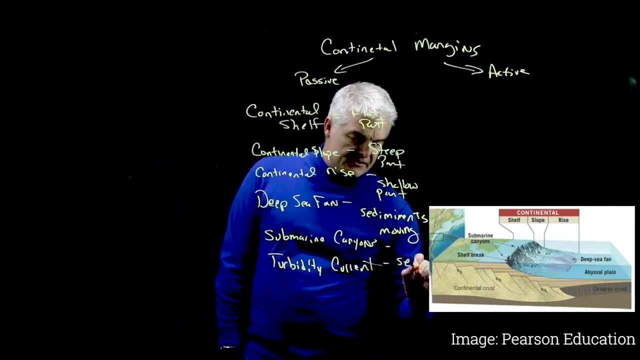 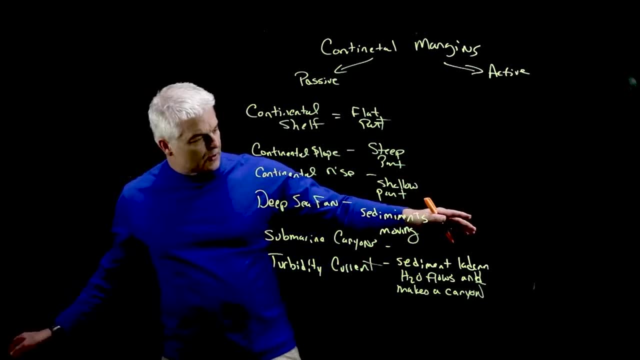 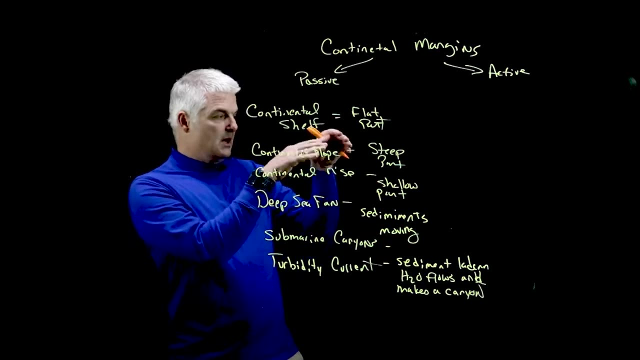 And this is when this Turdidity. It's only the third word. There's a second word opening the first one down, We'll see Limited water, Settlement-laden water flows and makes a canyon. Ultimately, folks, this is like mass wasting that we saw earlier in the course, where it 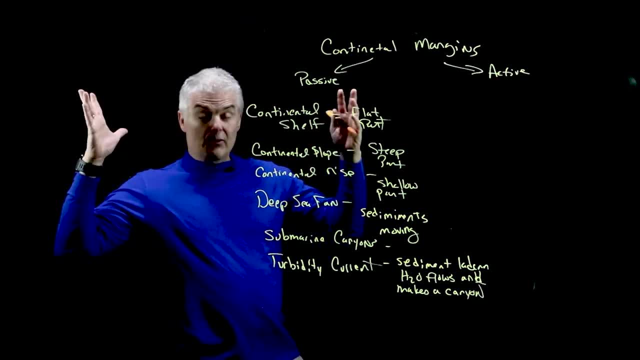 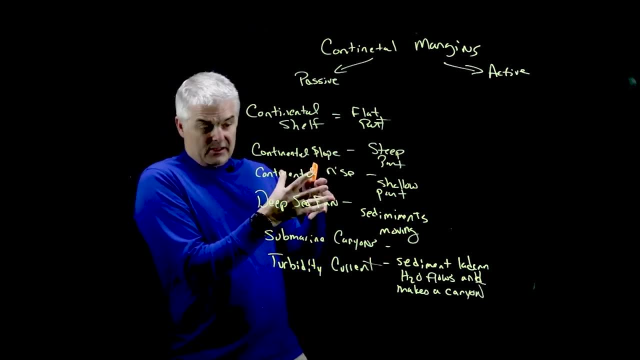 flows. When we talk about mass wasting, we just say there's a big rain storm and it causes this big thing to happen. Now this is all happening under water, so there's already a bunch of water. so the water is going to saturate the soil, the currents, the sediments, all the stuff, and it just 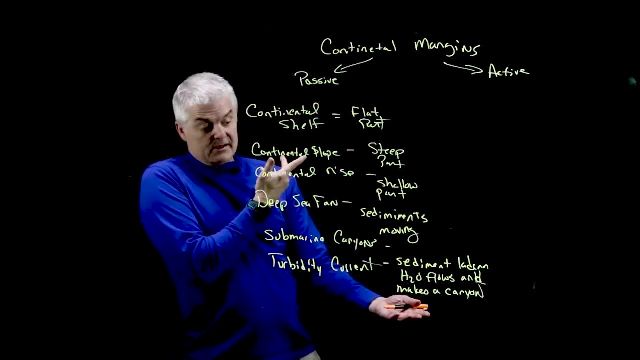 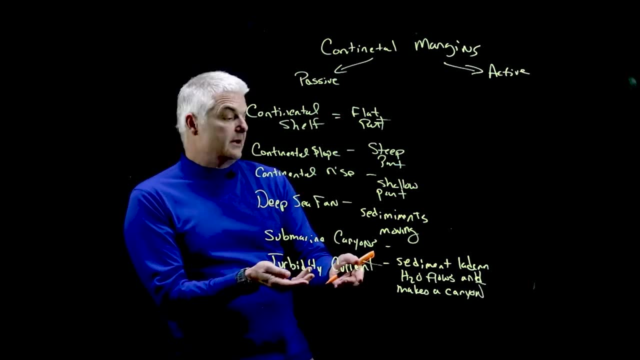 boing, just boom. It's looking for like a weakness And once it's weak, it just keeps going And you can have these really cool submarine canyons that are caused by these turbidity currents, And then these sediments. they go all over the place. We'll talk more about sediments and where they're headed. 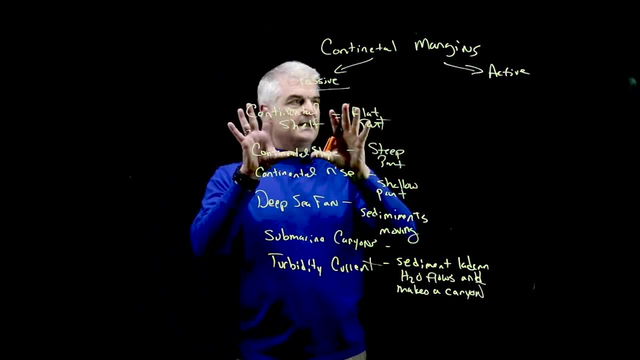 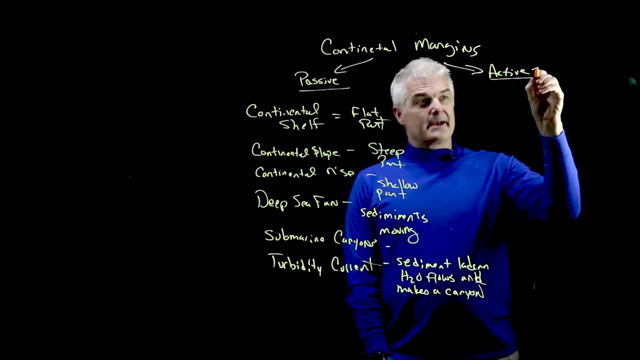 But yeah, passive plate boundaries. Now let's flick over and now talk more about active plate boundaries. Now, active plate boundaries as it makes sense. Now, when we talk about active, we're talking about active from a plate, tectonic Plate, That's an L 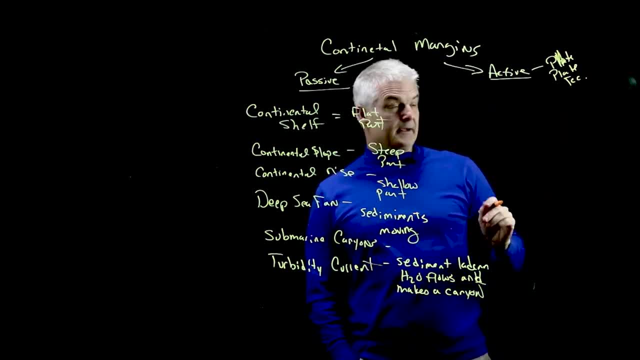 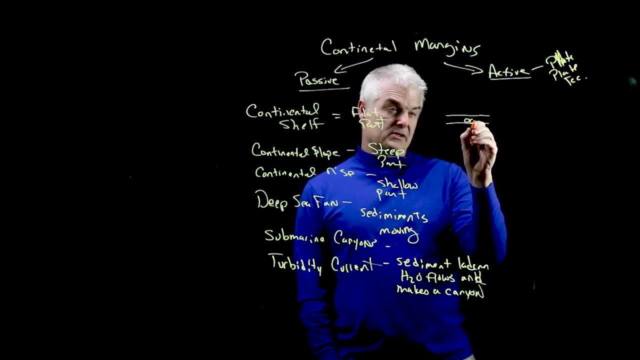 Plate, Tectonic, perspective Plate tech, And we've seen these before, right. So I've got two kinds of situations. If I've got an ocean- we're talking about the ocean, right, It's an ocean plate, And if it's heavier, it's going to subduct over another. But if I come in contact, 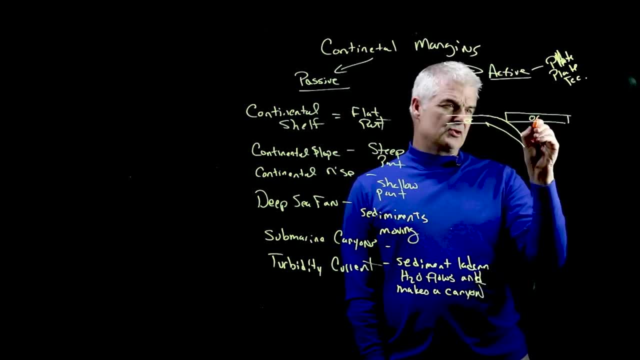 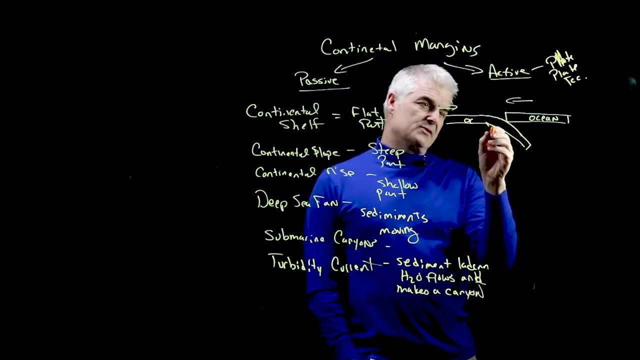 with another oceanic plate, right. So this is another ocean, Now the older one, 10,000 feet. So it's going to subduct over another. So it's going to subduct over another And they're moving in a convergent manner. And remember, what's happening here is this: 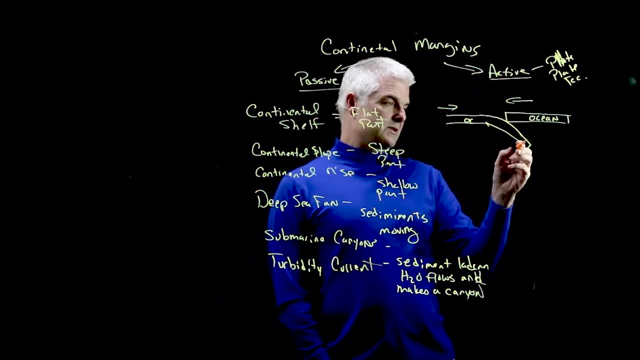 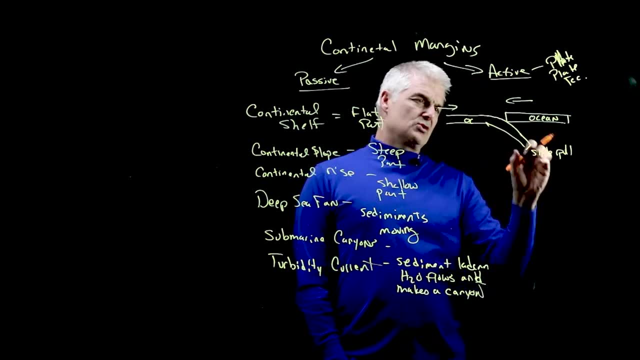 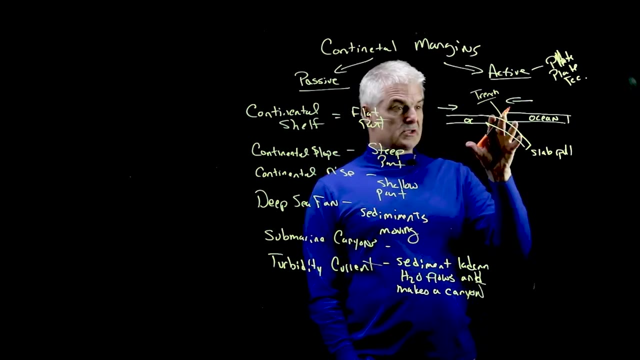 happens, One of the reasons it's causing this- we've talked about convection cells, but also just the weight of this- We call this slab pull, if you recall. The weight of this- just drags it and drags it And as it drags it, it often will make a trench, A deep ocean trench. 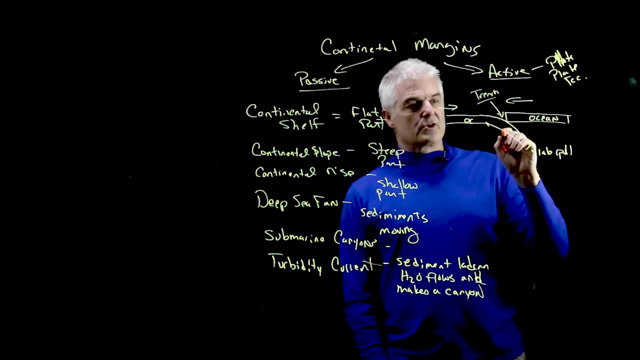 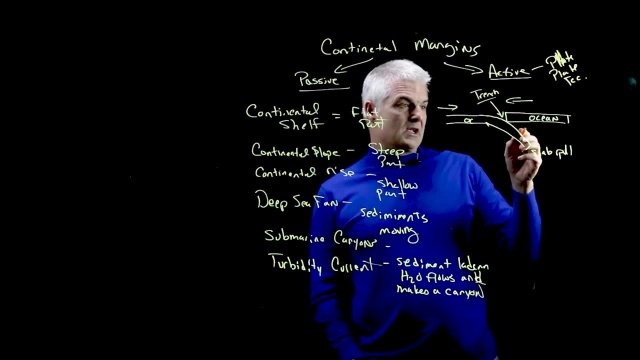 This is where that challenger deep that we talked about in a previous video. that's where you get these trenches And this looks like one little spot, but it's going to extend And it's going to extend across hundreds, thousands of, even miles. when they come across, Just get a trench, But 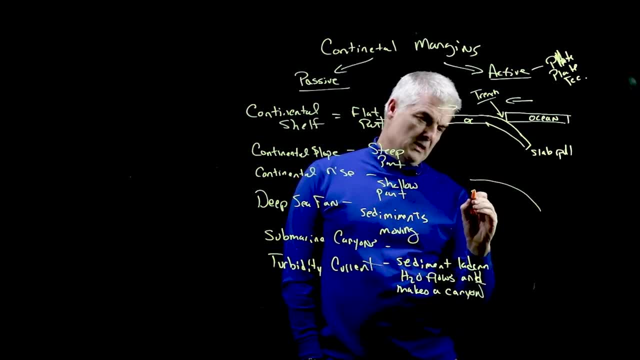 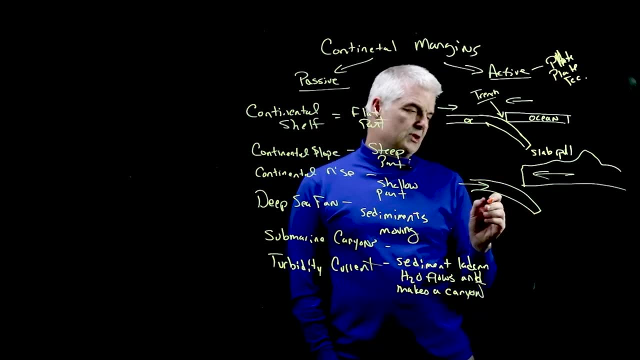 another thing that can happen. when you get an ocean- all right, an ocean. Now he collides with a continent, a big continent plate, Again a converging plate, boundary. You get something super cool And it's called- I'll misspell it right- an accretionary wedge. Let me write this: 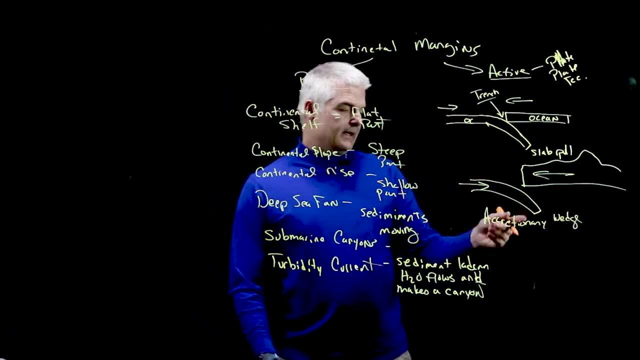 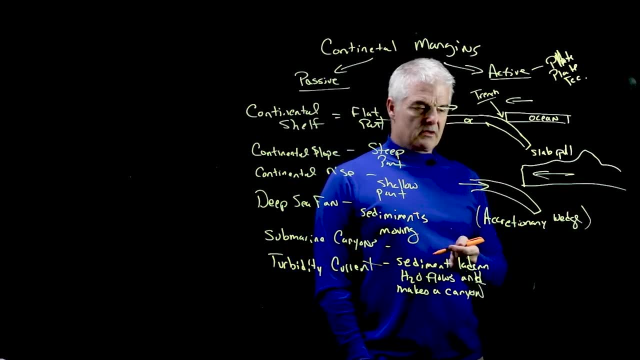 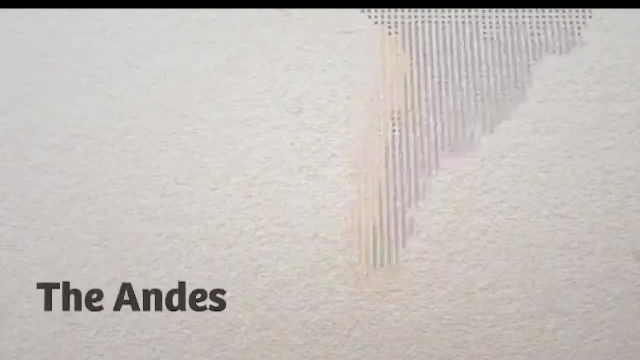 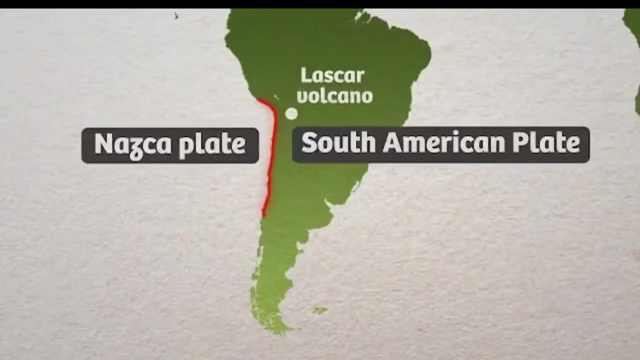 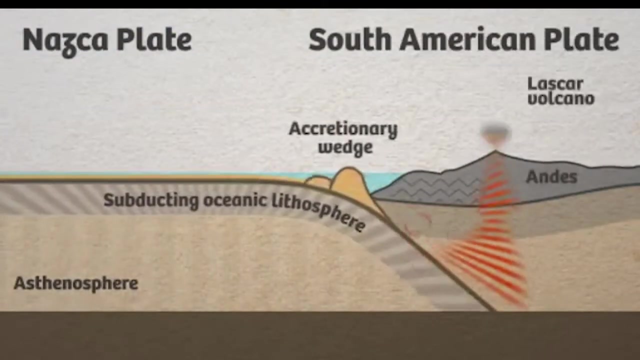 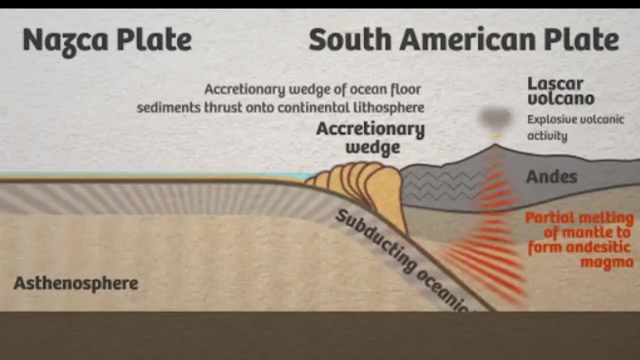 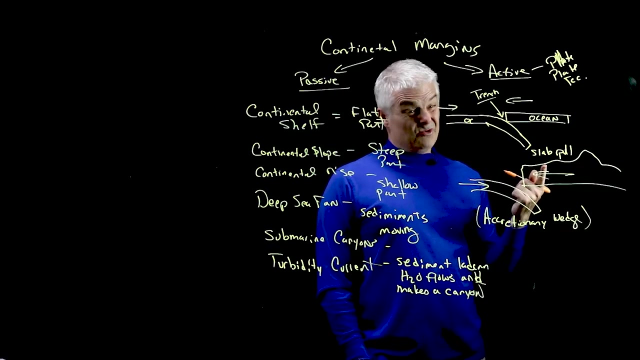 down And I found a video On YouTube, So let's play that video that shows us how an accretionary wedge works. That's pretty cool, But you see, what's actually happening is that as this collapses with or collides, it starts to fold this up And you don't actually get a trench, but you build up a new. 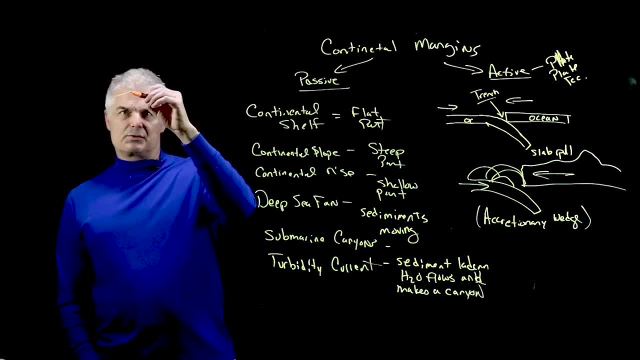 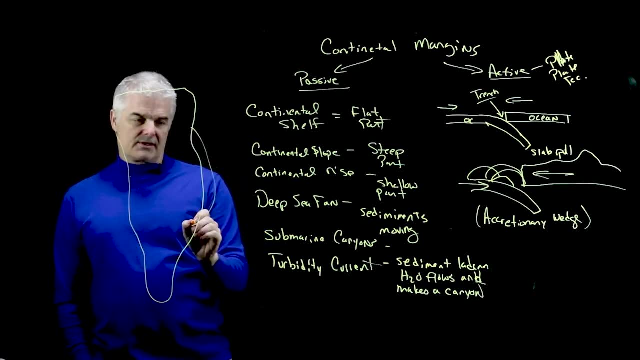 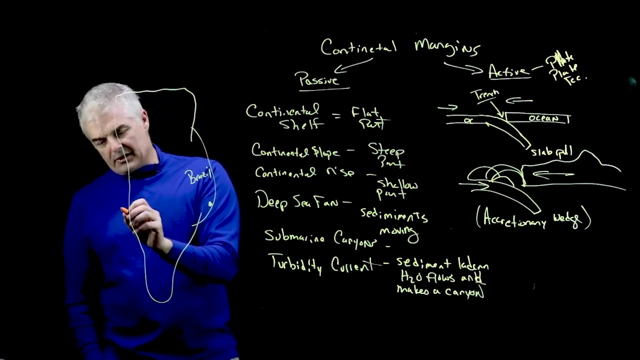 continent. You know an interesting place where this has happened. I've had a chance to visit this place. I'm going to maybe do a horrible job. This is an attempt to drive a continent- South America. There we go. This is Brazil, Rio de Janeiro, here, But anyways, we're looking at this. 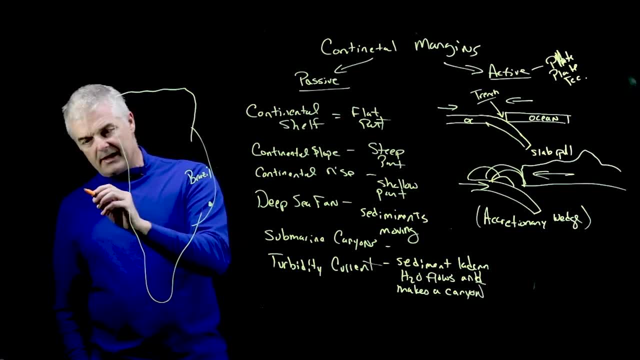 part. This is the west coast right here, And right here we've got the Nazca plate colliding with the South America plate, And you may not know this, but there's the Andes Mountains. some of the tallest mountains in the world are right on the edge, But you have an accretionary wedge happening. 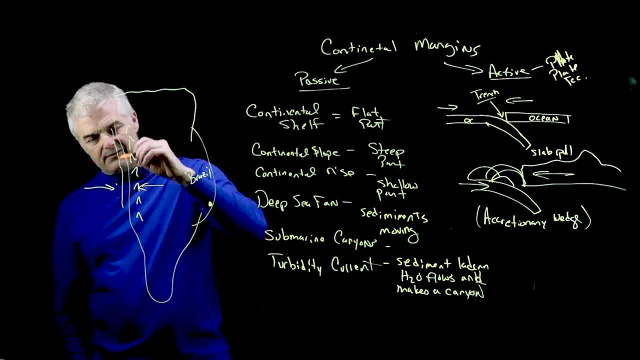 right here And it turns out that there's kind of a big flat space right on the edge of the mountains And this is all in a accretionary wedge. And if you dig down deep, if you will, what you'll find here is you're going to. 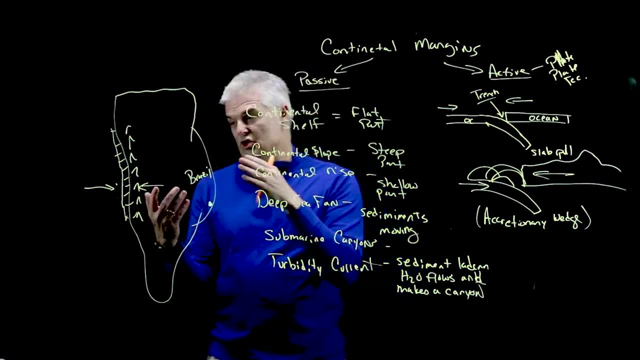 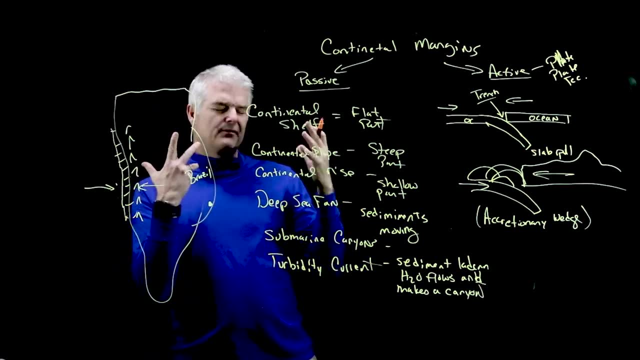 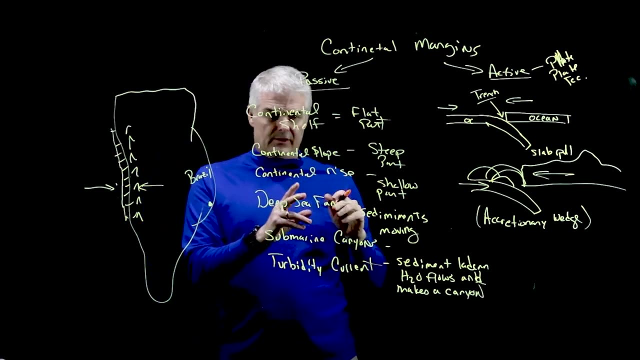 find seashells And ocean. what used to be under the ocean has been folded up, as we saw in the video here. So continental margins have an interesting. you know it's at the edge right And we've got the passive stuff with the cool picture and rises and runs- not runs- I'm too mathy. Rises and slopes.